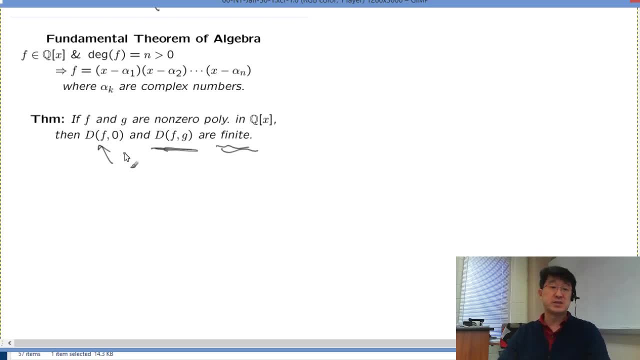 just one polynomial as long as it's non-zero, and there are only finitely many divisors in there, Why You can use something called fundamental theorem of algebra or unique factorization property. It seems like it's not so simple to explain why this is so, But I'm just declaring: 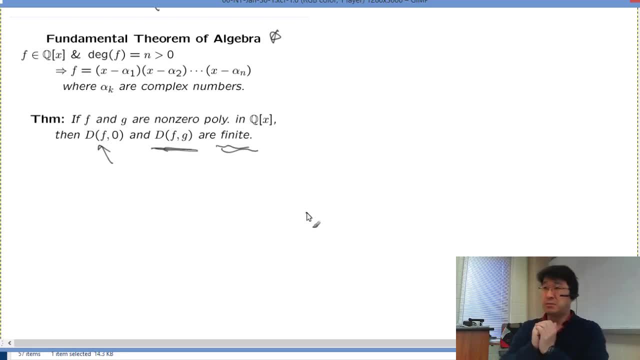 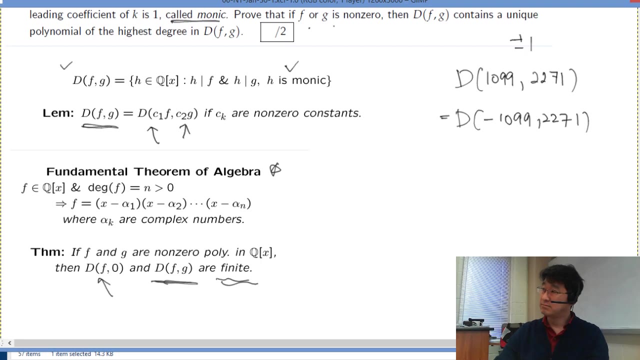 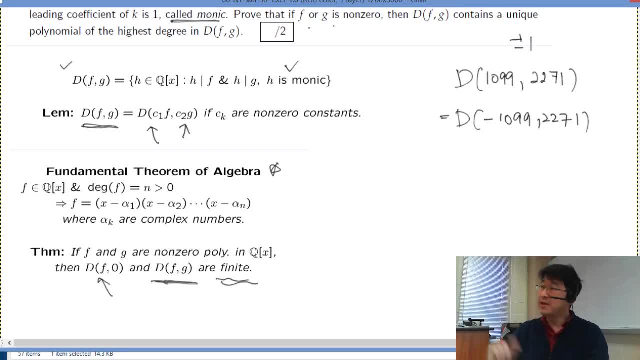 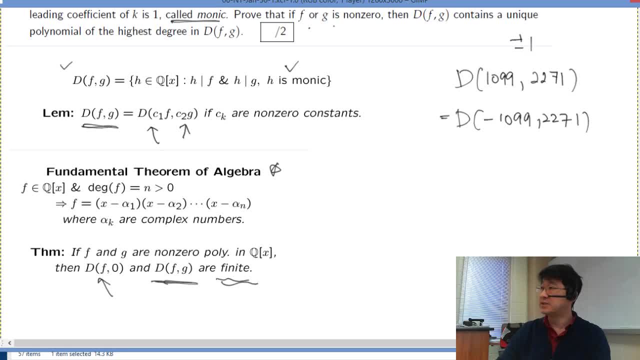 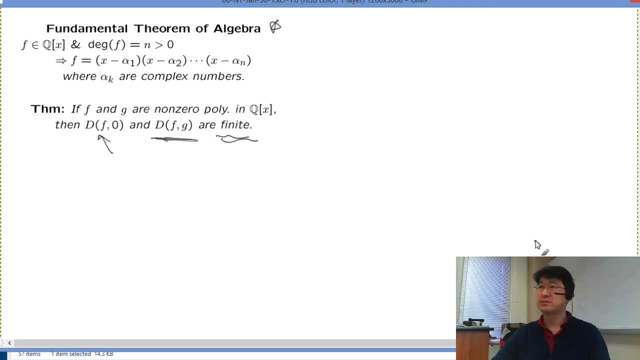 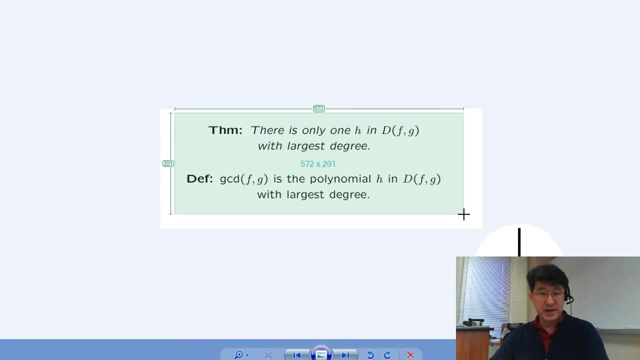 Not number mod polynomial. Yes, That works. Yes, Yeah, Which it was actually Euclidean algorithm. So it does work. Yes, Okay, Anything else. But we also saw that as a homework problem, that I just explained all this thing as a homework. 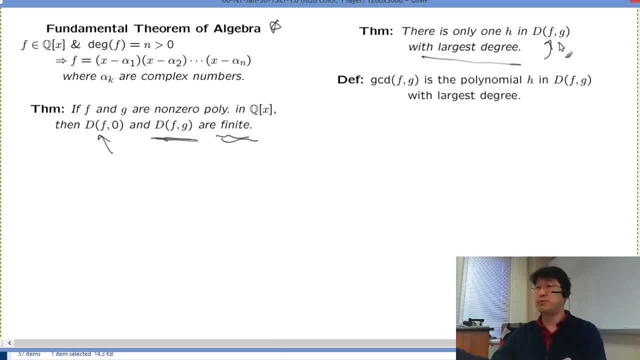 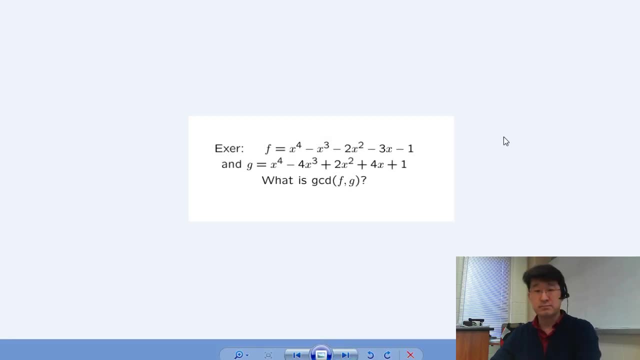 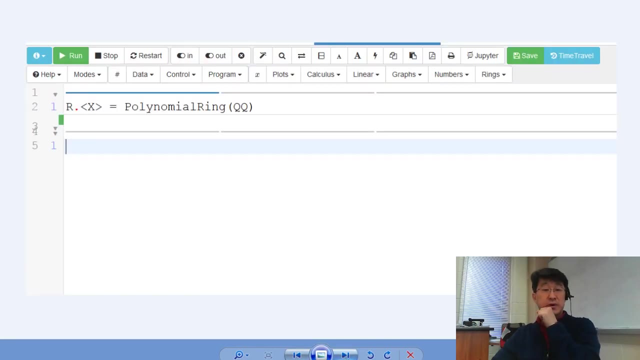 And there was only one polynomial with the largest degree in there. That's what we really care about, And that is the definition of a GCD. yes, it's also in that slide, so, um, that's what is. that's what you wanted to copy down, okay. 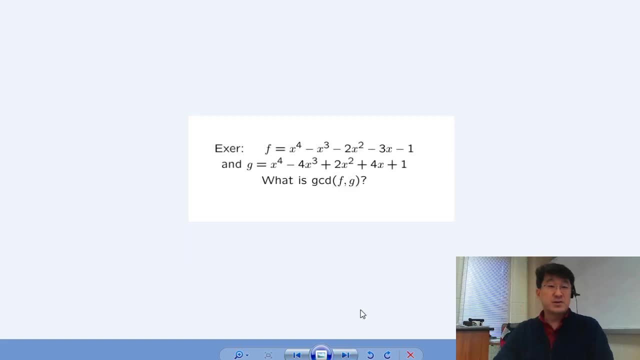 good, all right, all right, just like the homework problem. no one wants to divide this one by hand, and because you know how to divide one polynomial by another, we need a calculator, right? you don't want to, you know. multiply four digit number by four. everybody use a calculator, so number. 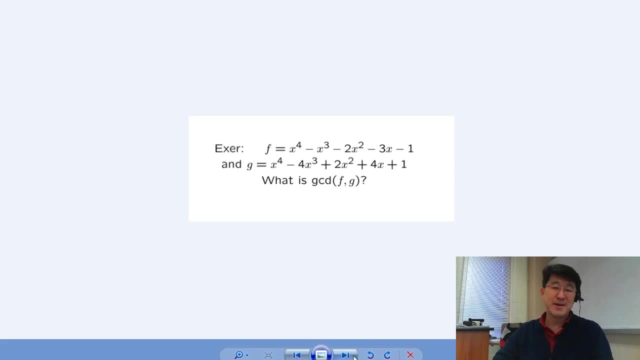 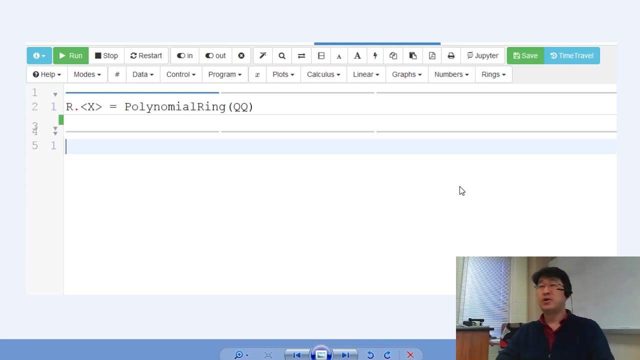 theory calculator. we need it, number theory calculator, and that's this sage. so we're going to start one at a time. this is a very simple thing i'm introducing here. all right, you want to declare a polynomial variable to the sage, and this is how you do it. 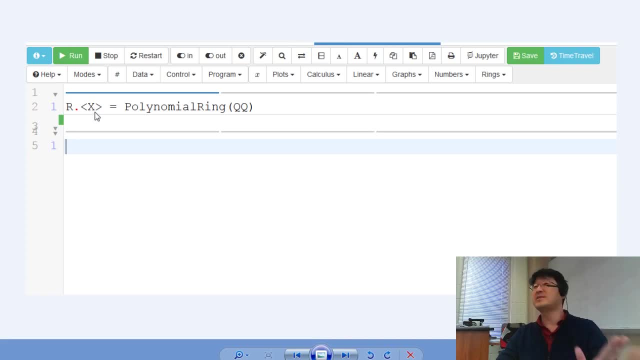 r is a ring dot x. x is going to be the variable for the polynomial. that's going to be the polynomial ring with a qq. it's a rational coefficients. now the sage knows that x is the main variable for the polynomial ring with the rational coefficient, so whatever. 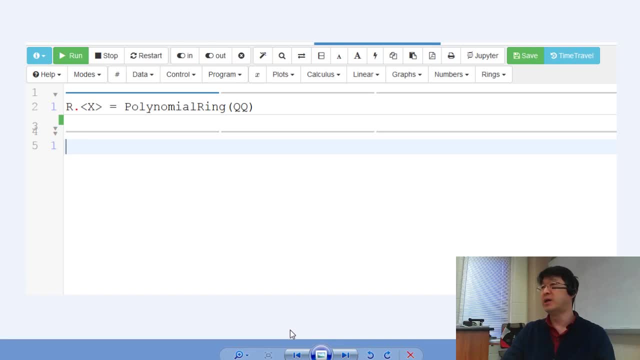 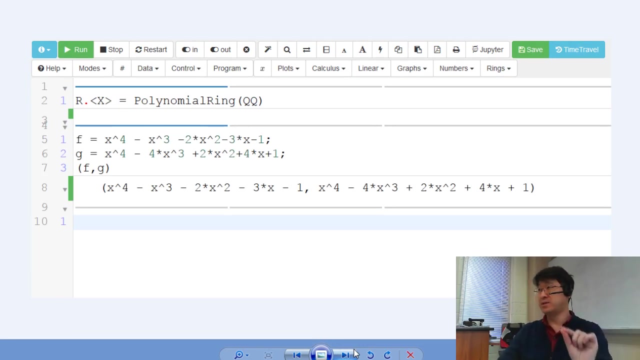 you write down with x in it, you recognize a polynomial variable, not unknown, not the you know usual computer, a variable. this is indeterminately recognized, so and you can define f like that, without parentheses, x like that. that's how we recognize f is not a function, it's a polynomial. f is just declared like this: you have to use a star in sage, it's. 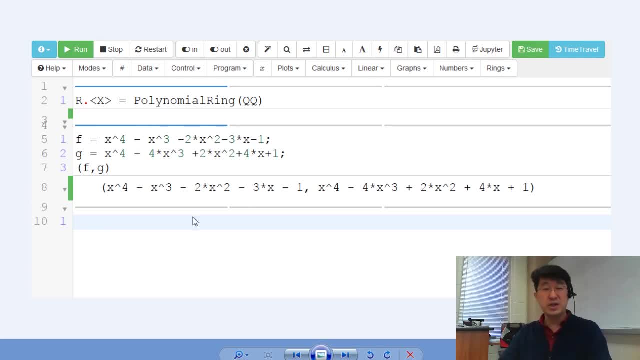 a python based language, so you must use star and g like that and f comma. g is just checking that if i entered it correctly or not, and then it spits out like that. so i check that i entered it correctly by returning these to us. it's not multiplication, this is just a random variable and all right. so 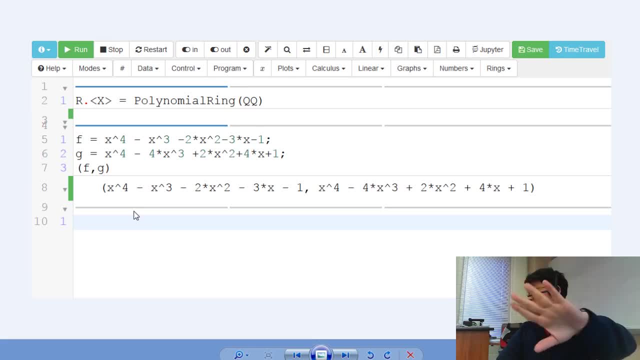 This f comma g. it's just state f that I just defined, and g separately. It's just like 3 comma 4.. It's just repeated exactly what I typed And one way- usually I do that if I typed it correctly, to check it. 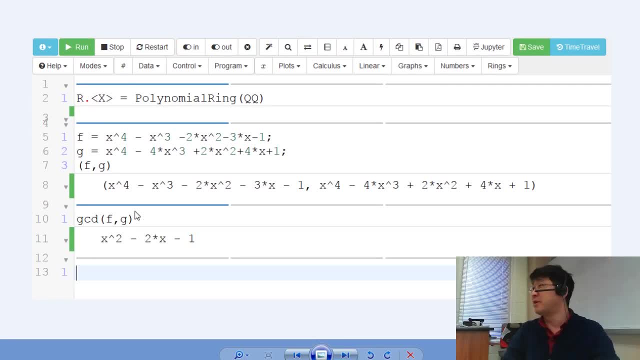 Then you just go ahead and write down gcd and it'll find the gcd for you. But we just spent some time to understand the meaning of this gcd of two polynomials, right? So it does it for you like that, So you can check your answer. 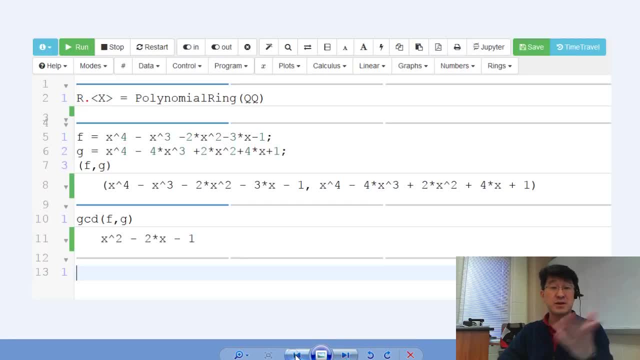 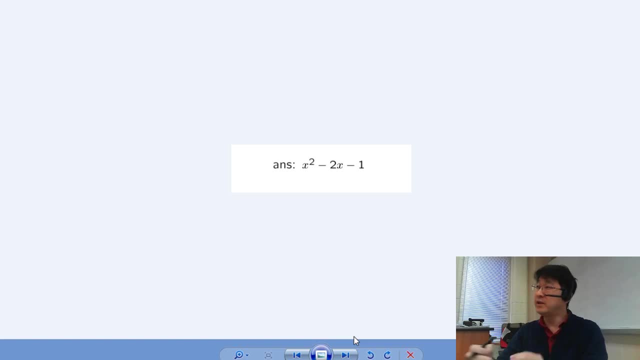 Good, And because of that the answer of gcd, of these two polynomials, x squared minus 2x minus 1.. But how do you do that in the test? You keep dividing one polynomial by another until you reach zero And whatever the other guy adds, change it into monic and match it to gc. 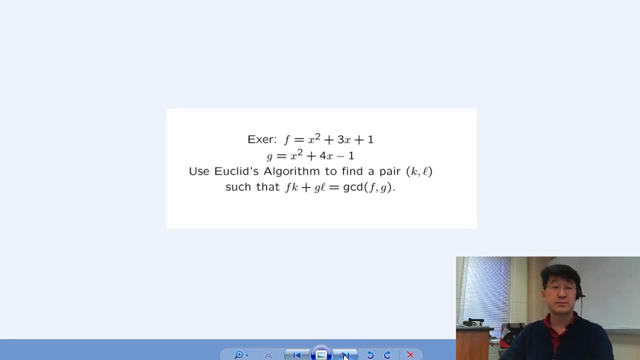 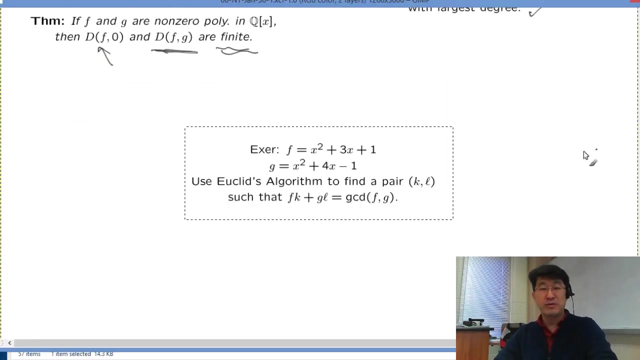 Good. So this one Is really simple. Why is that simple? Because it's degrees two right. Actually dividing is not painful. It's a really pleasant experience, All right, So we will do that, All right. Gcd is actually simple because you know how to factor this quadratic polynomial right. 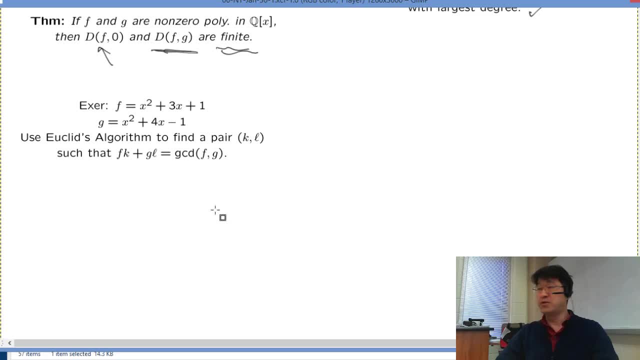 Because of that, this answer is in front of you. So our main goal is to get into that shape Right, But apply the Euclidean algorithm. get gcd figure out Bezou's identity Degree three or higher is pretty painful So I can't do that in the test. 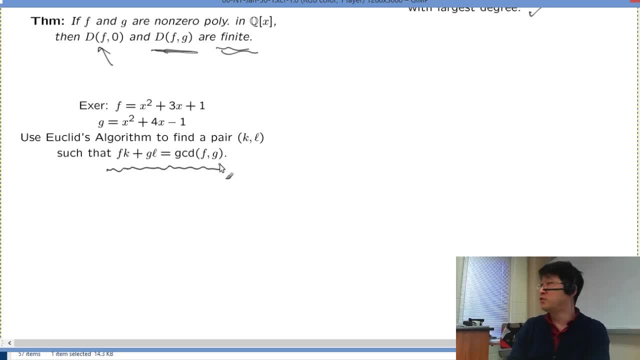 However, this is okay. So stick to this algorithm, Don't try to figure out other slick method. just to answer: two degree, two degree, two case. This exercise five. Am I counting correct? Okay, So, Chester, this is really simple. This 這就是不是 abducting the chicken. 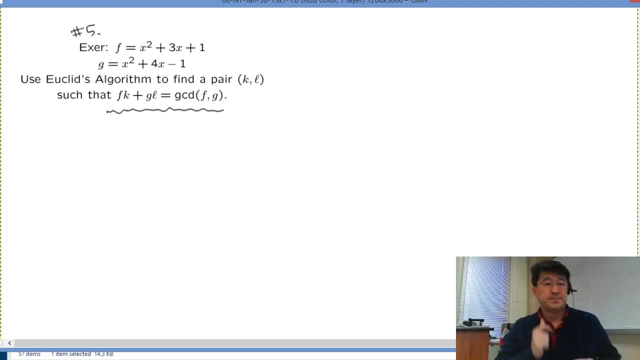 The more exciting one week. Thank you, No problem, You got this one. Thanks, You can play left. And that was just one guess, and this one that I chose I'm done here, So we will do this. I'm sure it's very hard. 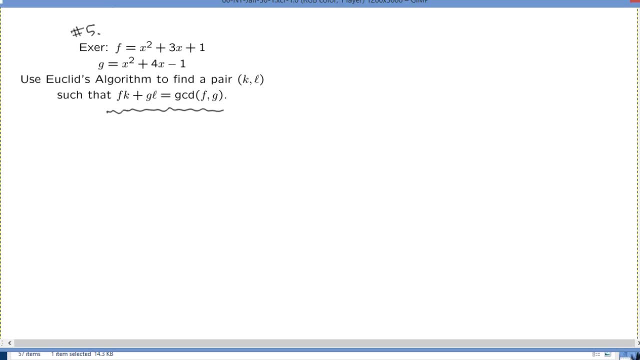 But I'm sure it's to work, this one. I don't see the X plus six because I like that X plus four. I'm kinda palliative malzu. x plus 4 divides that f. no, x plus 2. anyone else? what's it going to be? 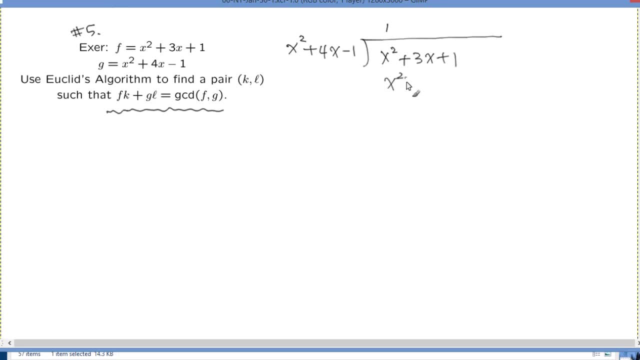 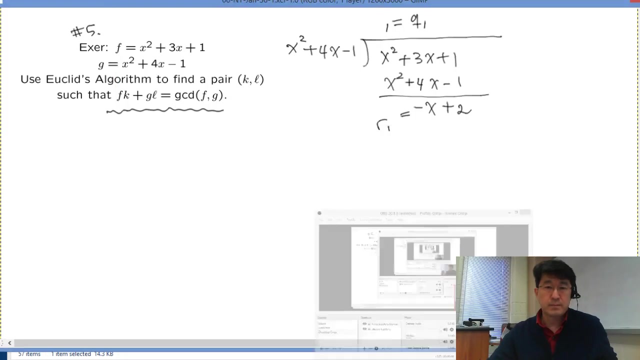 you, or how about doing like this? i can't do any other way when you're dividing two polynomials. this is how i do it, right, so i did it. and recording: i need q1, right, we're going to be using the q1 and here's the 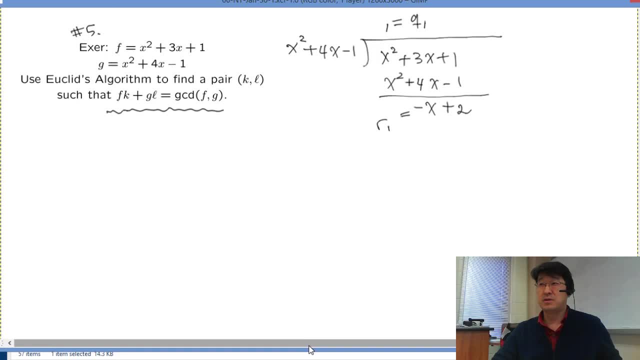 sinusoidal Philip speed r1. i recorded like that: make sense? do you know what to put in here? what are we going to divide next? r1 is going to divide g, right? so i'm going to put that g over here. how about that? g is coming over right, is that okay? and that's going to be q2 and whatever the remainder you 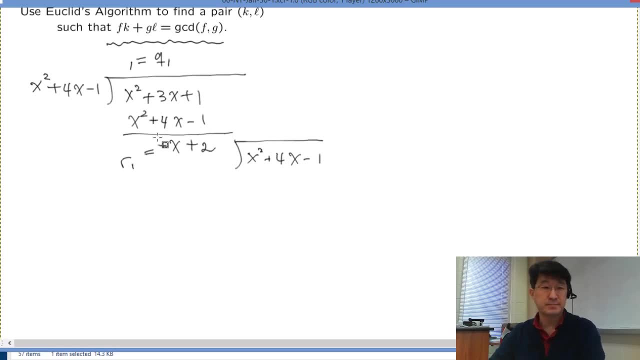 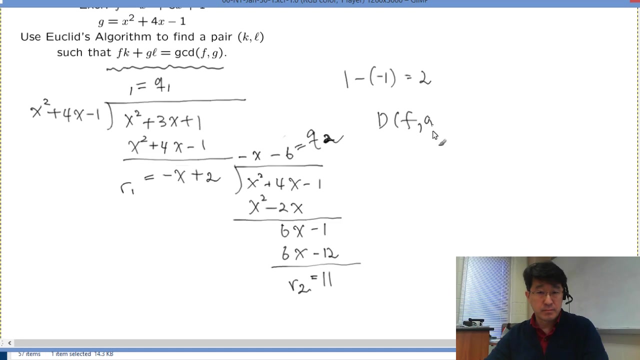 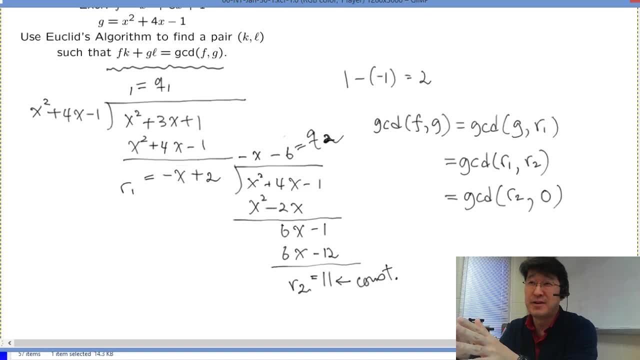 sure, like you don't want to make the mistake I made last time, make sure you enter the zero and clarify all that rather than this can use it, so it's not necessary if you know what you're doing. oh, I got constant there, I'll just stop. 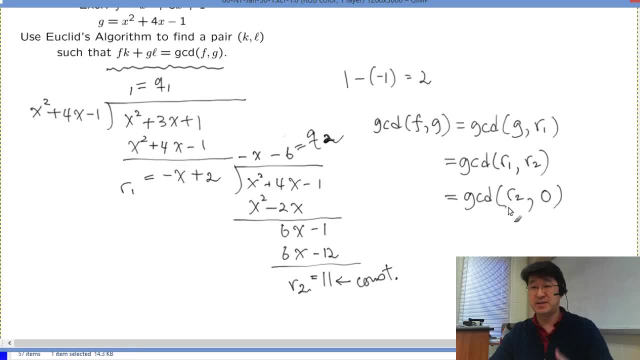 you, and that's my GCD. that's fine, but I did one more. if you divide any polynomial by kinds- constant, what is the remainder? right degree less than zero, negative infinity, right. so you had to enter zero in there. but that's just clarification. so do you have an answer? 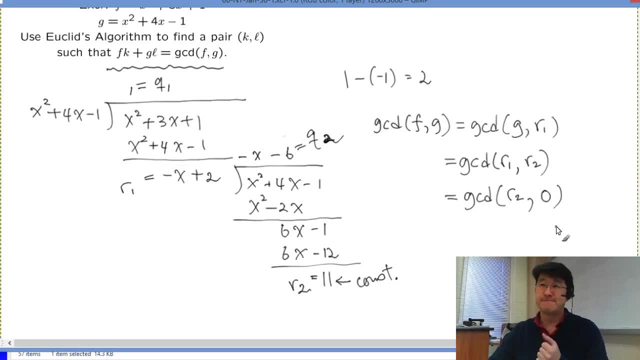 now, what is a GCD of these two polynomial? 11 is not the answer, but very close, almost. it's like 99%. what's that? no, it has to be monic. that's it. so what is the monic polynomial version of 11? what? what monic polynomial divides this? 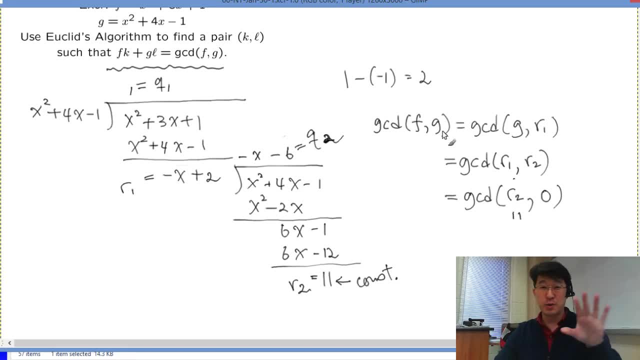 11 right. so monic polynomial, highest degree of monic polynomial, divides that the same thing as monic polynomial divides 11 and 0 right. what is it? 1? 1 divides 11 right as a polynomial and it's monic, but 11 is. 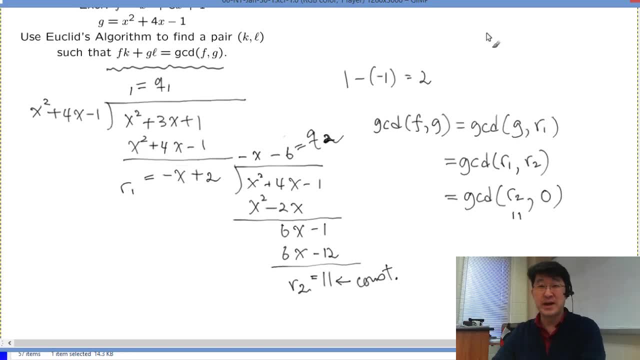 not monic. the coefficient is not. so if you end up 11x, GCD of 11x, like this, what is the answer? not 1, x, the monic version that divides 11 times x. Yeah, Monic polynomial. So the answer here is 1.. 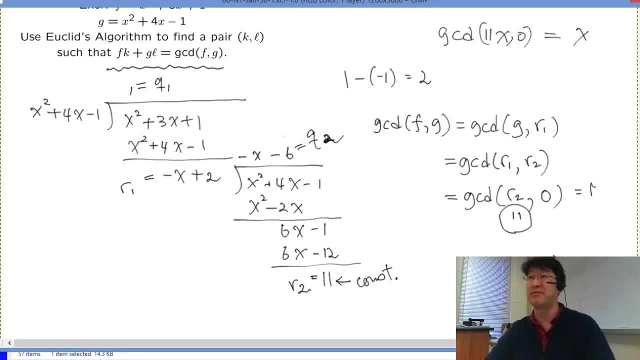 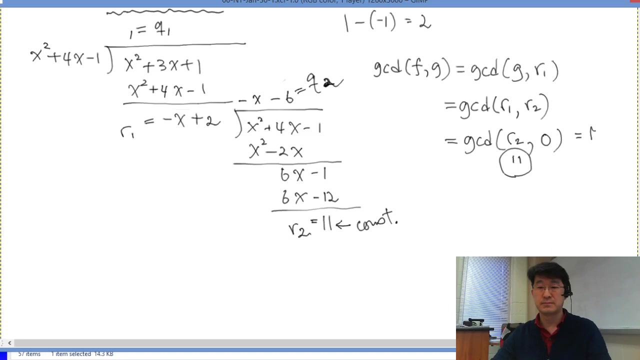 Monic polynomial that divides R2, which is a constant polynomial, 11, is 1.. That's called irreducible polynomial. yes, You cannot divide any further. called irreducible polynomial. These two are irreducible polynomials over Q. 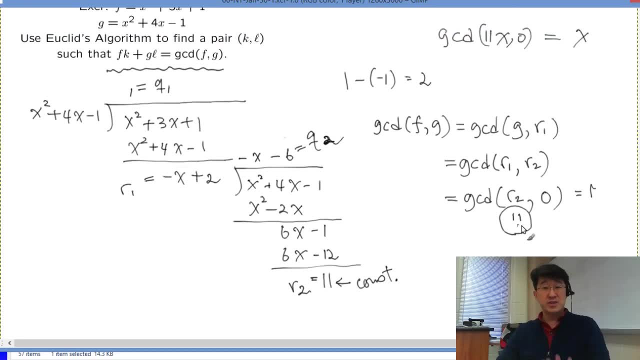 All right, That's that, but we can't change that 11 to 1.. You have to look at this chart- Q1 and R1 and Q2 and R2, as it is exactly, and you enter matrix version. Can you enter matrix version? 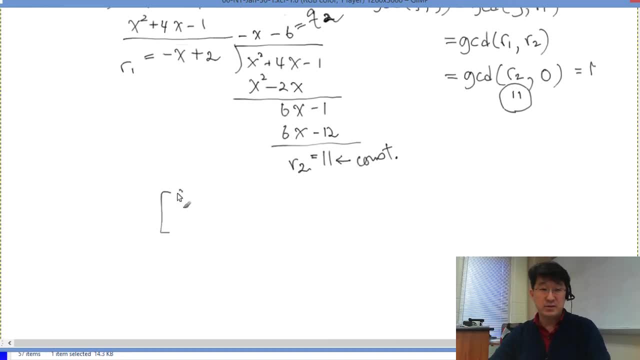 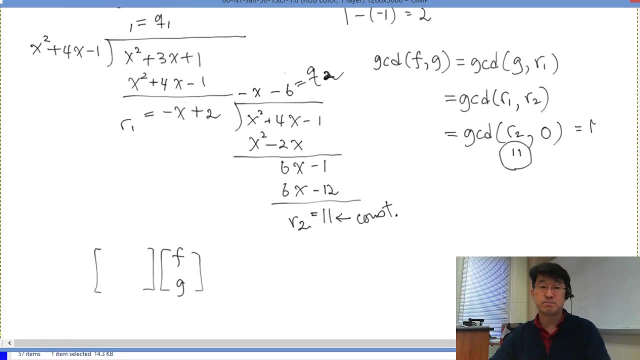 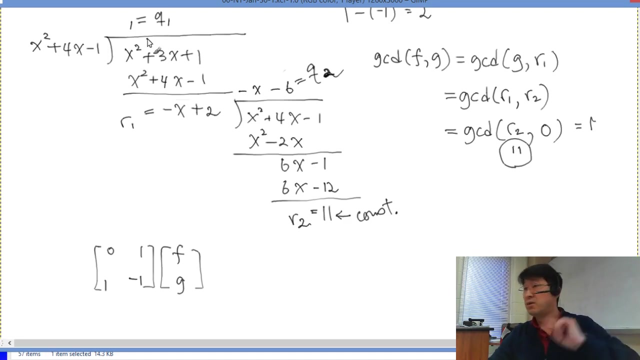 Start from f and g. right f and g are the degree 2 polynomial. What? What is the first matrix? do we have to multiply here 0,, 1,, right, 1, and what is the other one? Negative 1,, that Q1 in there? 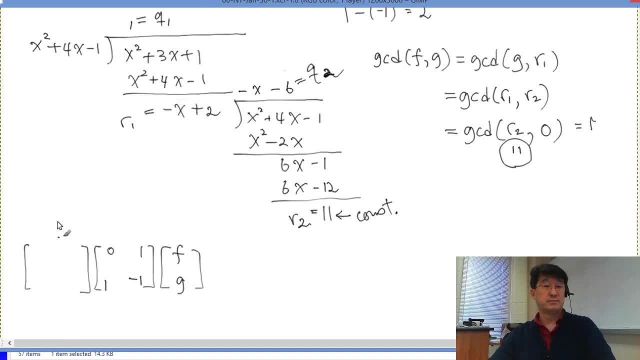 What is the second one? 0,, 1,, 1, negative Q2,, which is x plus 6, right, Yeah, And then by doing that, you're going to arrive here, I think. Right, R2, yeah. 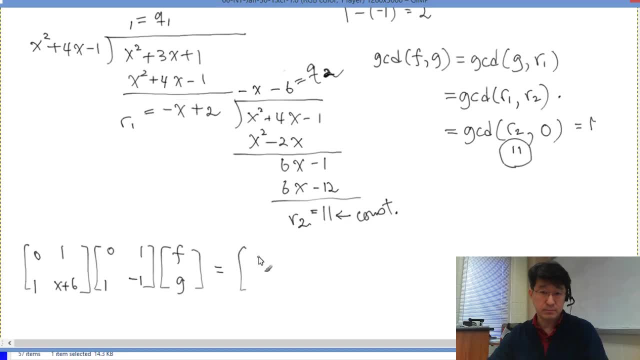 This is Q2, and it arrived in R2.. That's correct. yes, Is that right? Yeah, All right, We haven't reached the answer yet. This is what they're looking for: fk plus gl equals gcd, right. 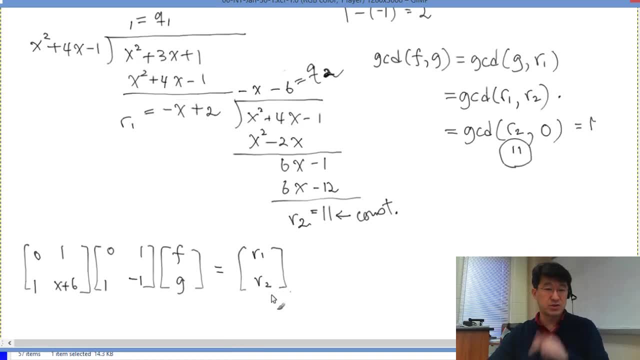 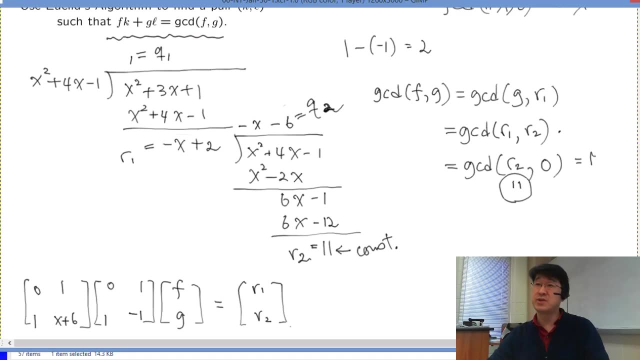 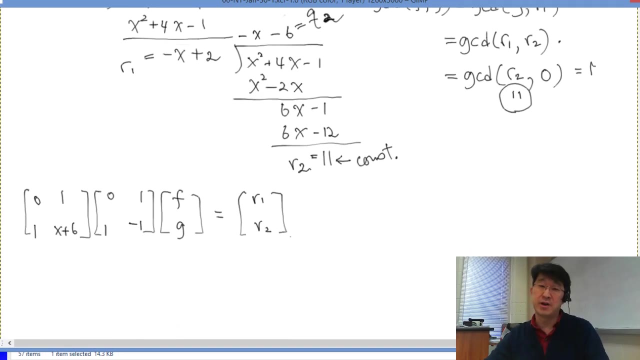 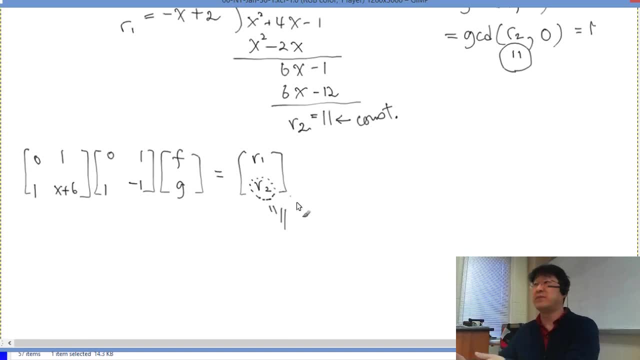 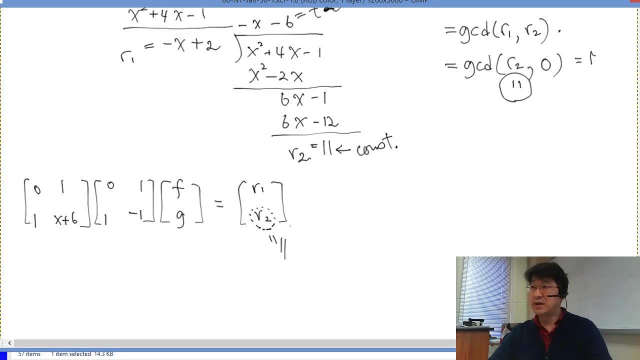 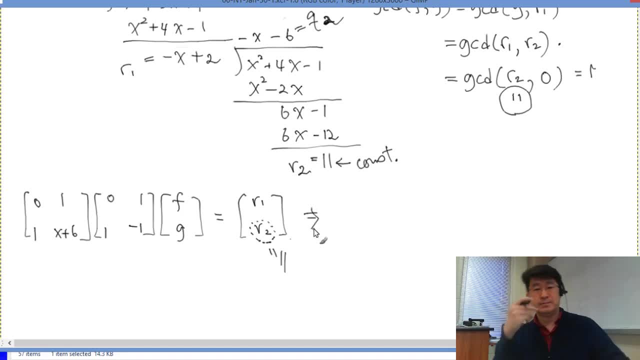 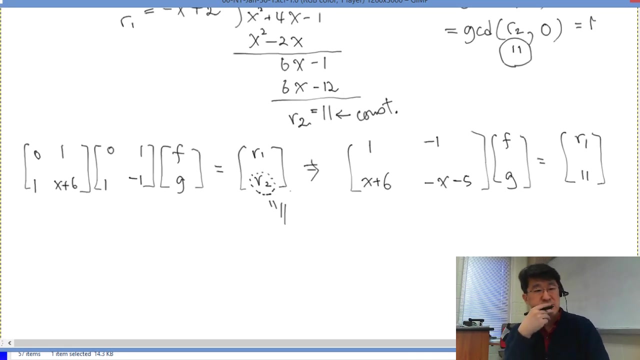 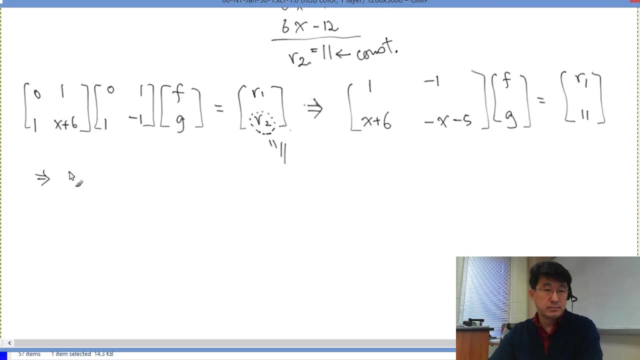 Write down what is 11, and see if you can actually gcd reach the gcd there. Thank you, Thank you, Thank you, Was that alright? Yeah, x plus 6 multiplied to f, to the degree 2.. x plus 5 multiplied to the degree 2g. 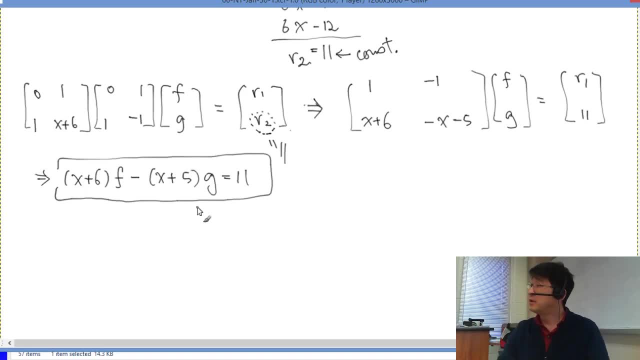 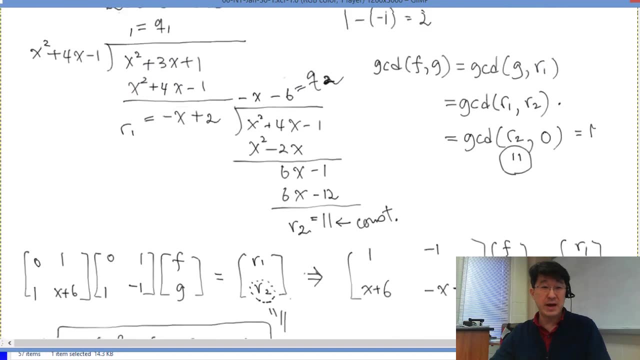 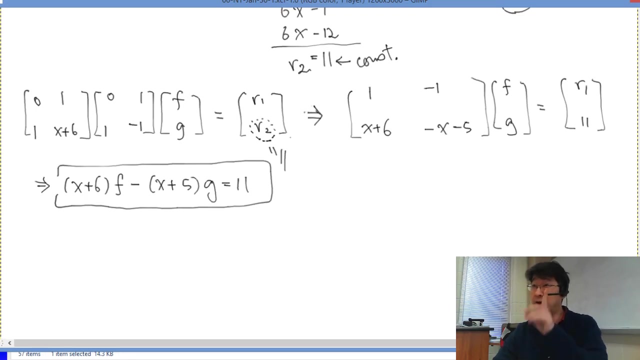 If you subtract that, all the x's cancel and give you the constant 11.. Fair enough, So did you realize that we haven't really reached that answer in there? fk plus gl equals gcd. What is gcd 1, right, So you have to divide everything. 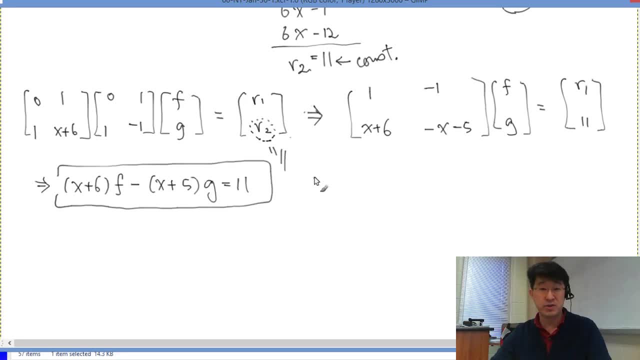 by 11.. That is the final answer. Then you reach there: 1 over 11, x plus 6, that linear polynomial multiplied to f, 1 over 11 multiplied to x plus 5, and to that quadratic polynomial. 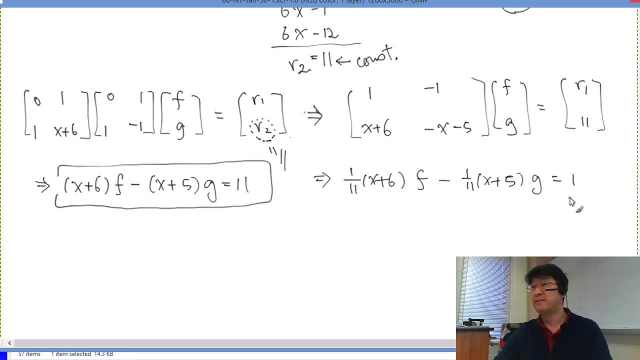 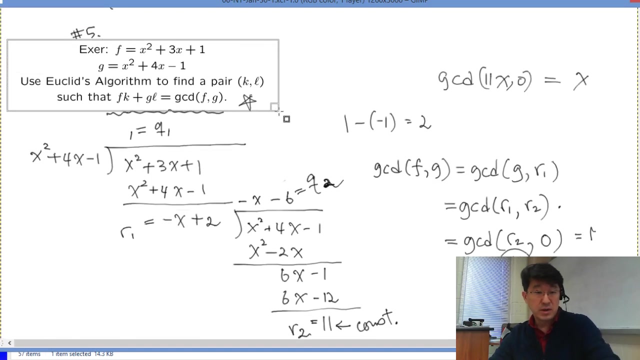 g now finally reaches this 1.. Man, this is a lot of calculation, But these secret functions that polynomial multiply to give you 1, are coming from this. All right, Let me go back and go back to copy that question and look at this answer and just compare that reflect on one more. 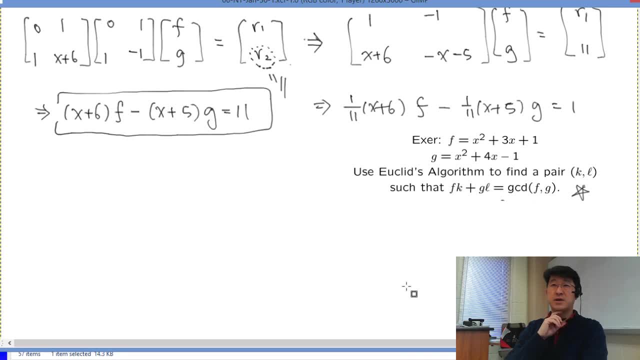 time. All right, That's how you do it. What is this statement called Perseus identity for polynomial- All right. Once you reach that, the integer version is like a real piece of cake. All right, All right. I have one more really strange exercise. 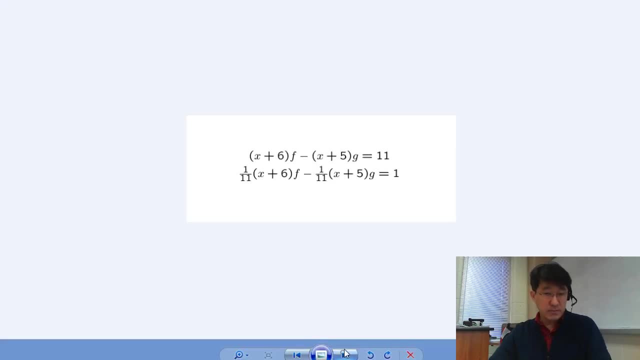 What will you do now, Jay? I'mlast thing to do is you need to call or put this table up and down For some reason. you want to simplify it. Say you know, you teach you need to write more functions For someone who's on the other side of the. 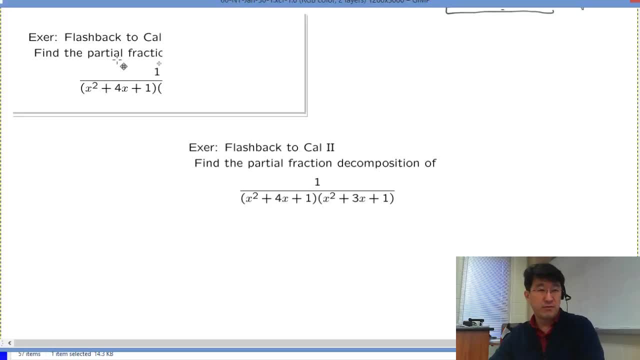 table. you can go either Or you have or you can see God do of you. I think I can't because I don't know about you. So that's the last question. That's next question. Now you're on the boundary, but you know what You're not doing: Yoursistan, You're doing. 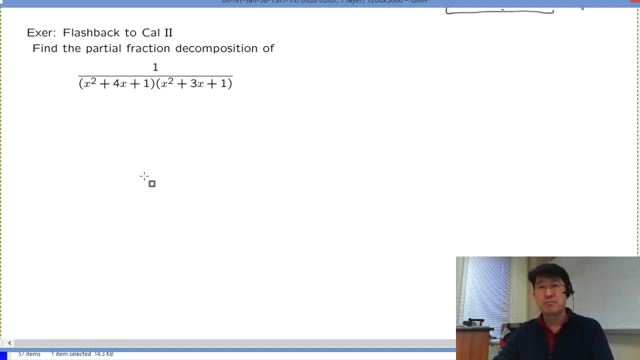 it right. If our total, how much you can apply this question is: why, but twice? right. The answer is yes, Yeah, partial fraction, decomposition of this. What is the hint? That's right. whatever we did has something to do with this one right. 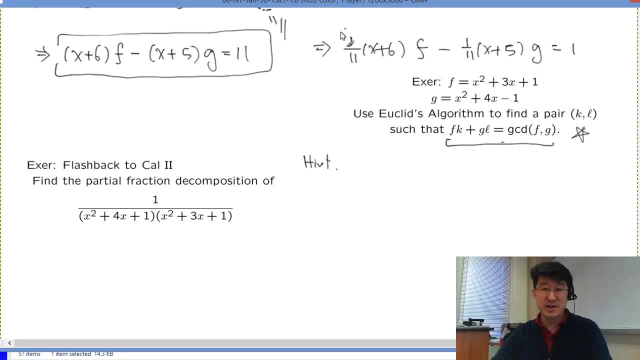 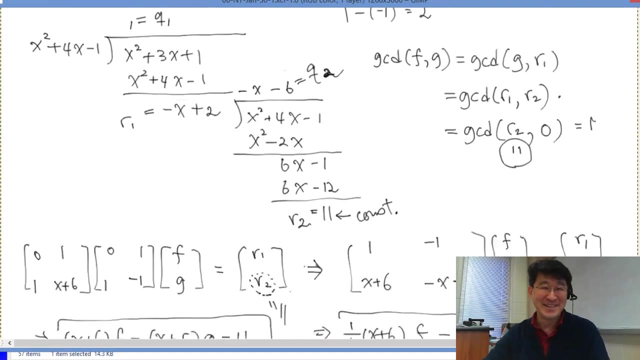 So I want you to go in and stare at this guy, stare at this guy really intensely and see what that is. That's our exercise number six. is that right? No, they don't see it. Don't tell them. They don't see it. 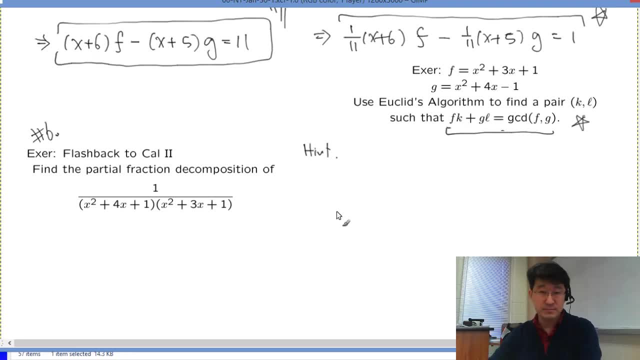 There it is, exercise six. All right, if you see it, do it. If not, keep looking at it until you see it. Here's a hint: That one and that one is the same one, right, That one and that one is the same one. 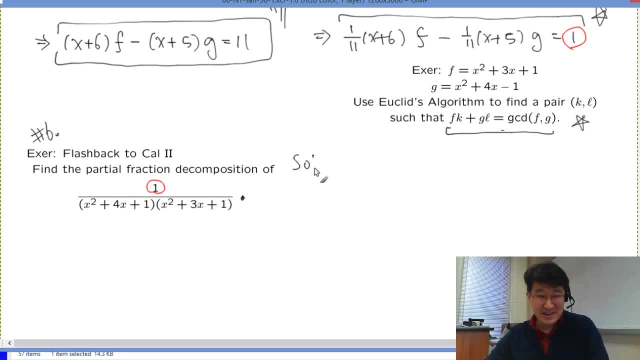 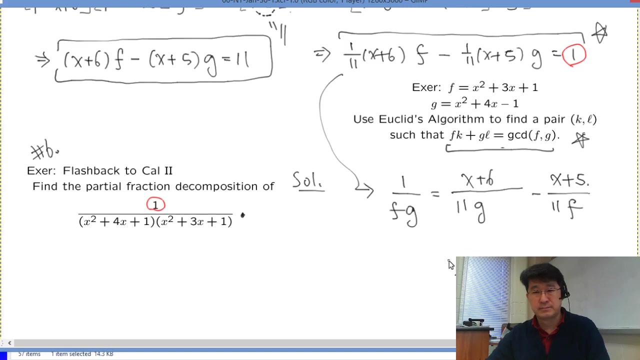 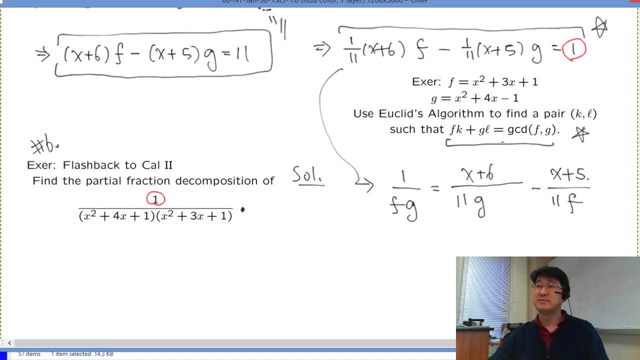 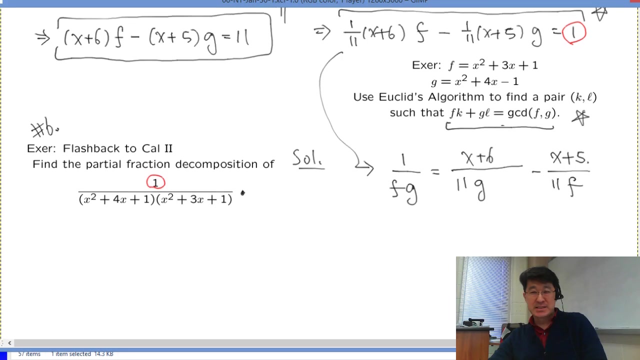 If there's a long division, it's not going to work. 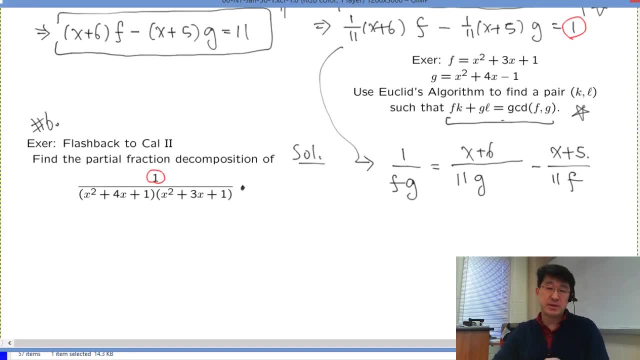 All right, That gives you another interesting statement. This is how we approach the partial fraction decomposition problem in Calculus 2.. You write this one like this. right Any question about my answer? You just divide both sides, f and g, and cancellation gives the answer. 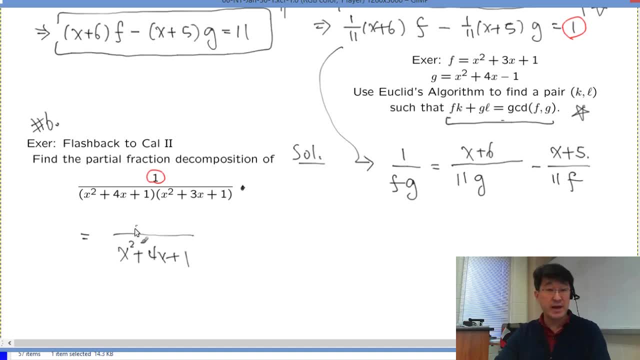 That's that. So it goes like this. right, And write down ax plus b, Remember that part- And write down x, squared plus 3x plus 1 and cx plus d. Now expand them out and you enter 4x4 matrix. right to solve this thing correct. 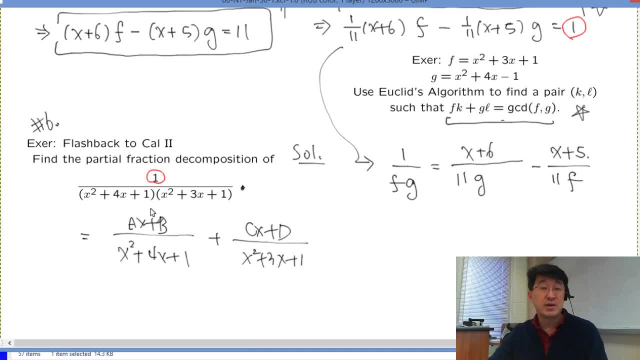 But if you think about the logic behind it, it goes like this: Suppose this is possible, Suppose this is possible, Then I will find a, b, c and d right, If someone asks you this question. why is this always possible? 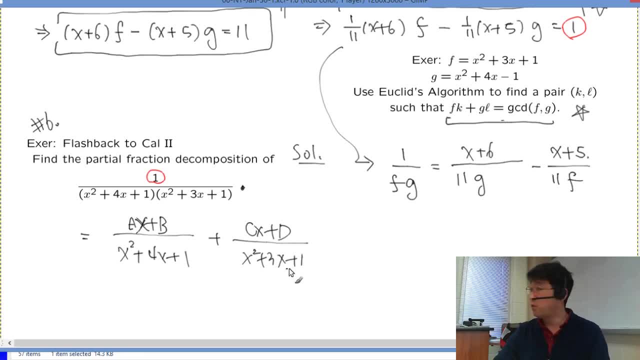 What if I have degree 2017, I overhear degree 275?? Why is it possible to find this? a, b, c? You look at this gigantic matrix, right? How do you know it's solvable? Uniquely right? 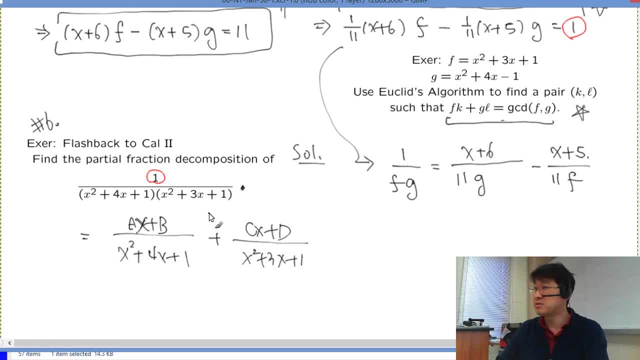 What is the answer? You know the answer: Bezu's identity. Because we show that it exists. right. Why does it exist? Euclidean algorithm gives you the existence of Bezu's identity. That gives you the solution to that problem. 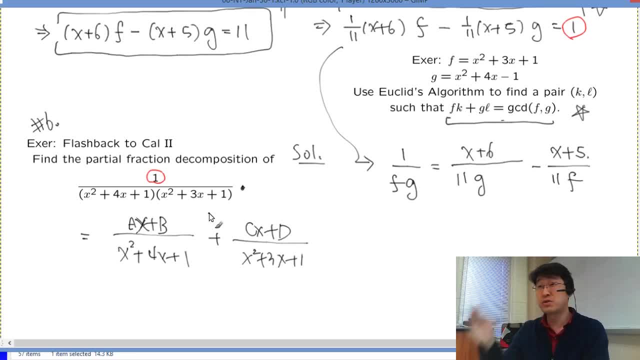 That gives you the existence of that, As you can see, is how profound this implication can be. If you're staring at this problem and look at that matrix, for example, if I play with the 3x3, you look at the 6x6 matrix, staring at that equation. 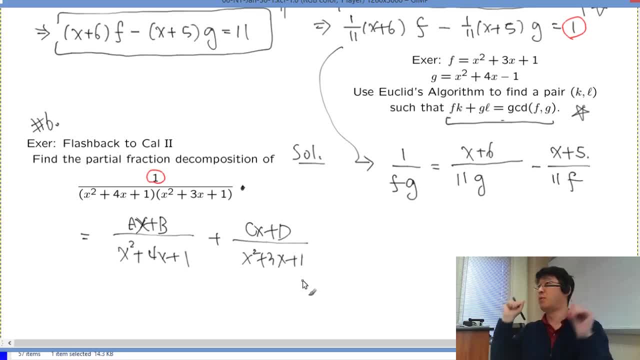 wondering why the 6x6 matrix is invertible. no idea really, But Bezu's identity says it's always solvable. Therefore it's unique. Uniquely, it's invertible, right? So even though it started out as really simple, 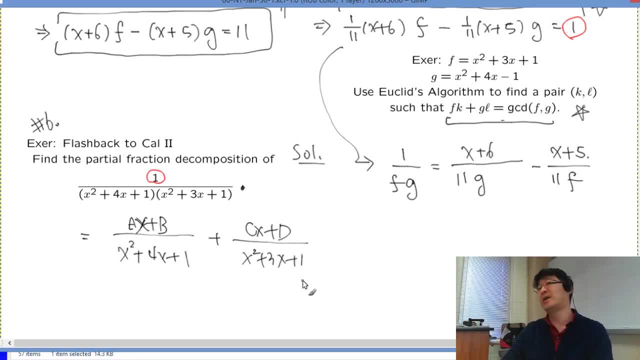 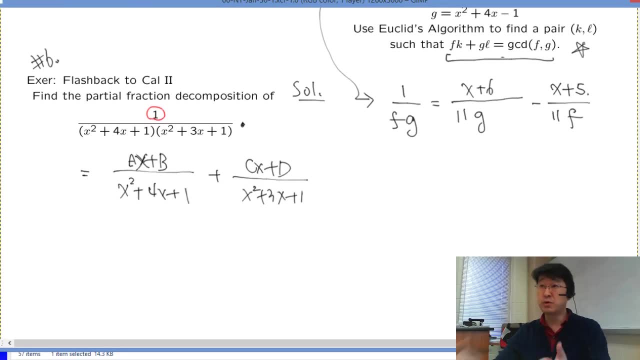 that you know like two or three line proof from Euclidean algorithm. it has far-reaching implication if you keep playing with it. So long division gives you the Euclidean algorithm. It's the coolest thing right. Worth spending time on this one and fully understand what goes into that. 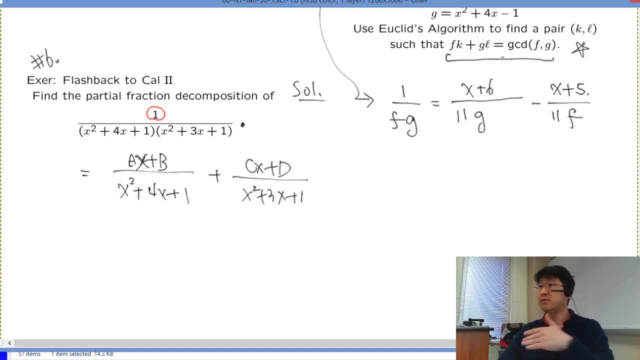 and what the implication is? It's still there. Still. it has more implication towards the unique factorization prime numbers, all coming from this Bezu's identity. All right, So I'll stop here today. 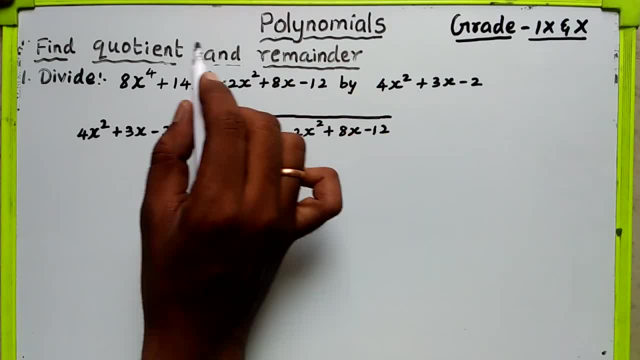 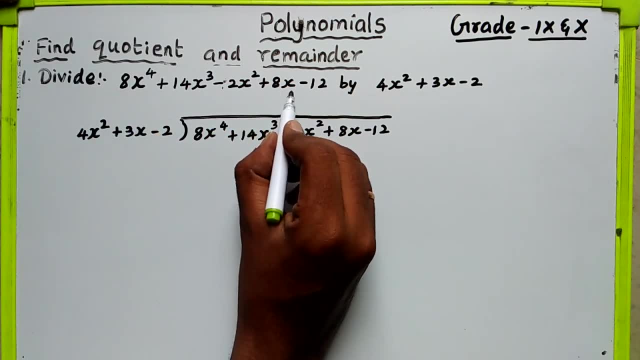 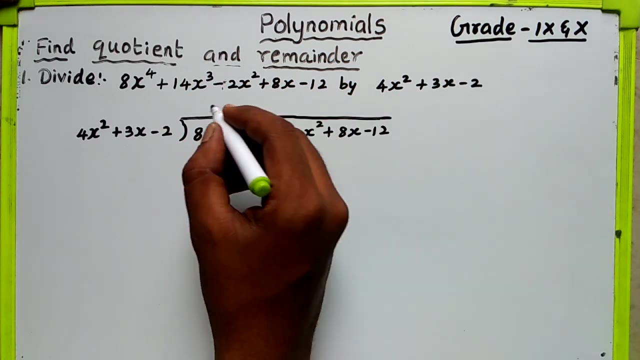 In this session. polynomials: find quotient on remainder: Divide 8x power, 4 plus 14x, cube minus 2x square plus 8x minus 12 by 4x square plus 3x minus 12.. Long division, I will take.